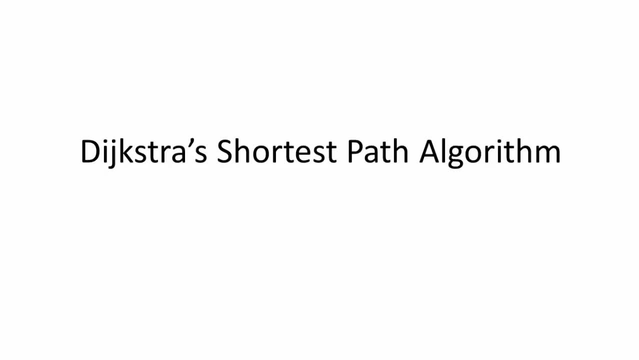 Dijkstra's shortest path algorithm was invented by the late great Edgar Dijkstra, a famous Dutch computer scientist. The objective of the algorithm is to find the shortest path between any two vertices in a graph. In fact, Dijkstra's algorithm will find the shortest path from a given starting vertex. 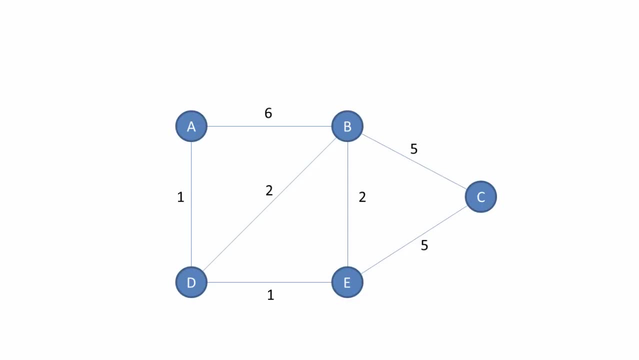 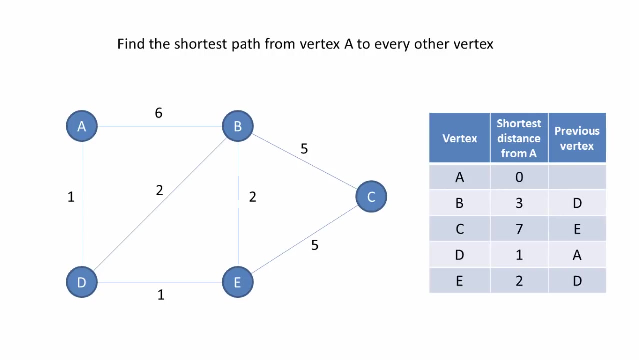 to every other vertex in the graph. Consider this simple graph. Our objective is to find the shortest path from a to every other vertex. Once it has run, Dijkstra's algorithm will generate this information, which includes everything we need to know. We have the shortest total distance from the. 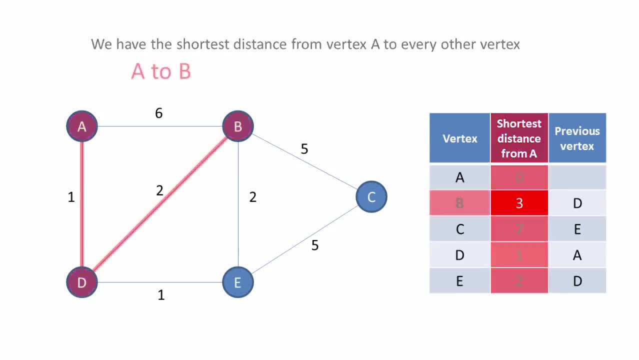 starting vertex to all of the other vertices. The total shortest distance from a to b is 3.. From a to c: it's 7.. From a to d: it's 7.. From a to d: it's 1.. 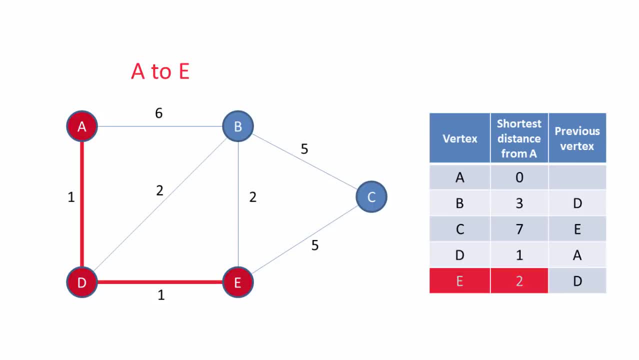 And from a to e it's 2.. We also have the shortest sequence of vertices, from a to every other vertex, In other words, the shortest path, For example, to get from a to c. notice that we arrived at c via e. 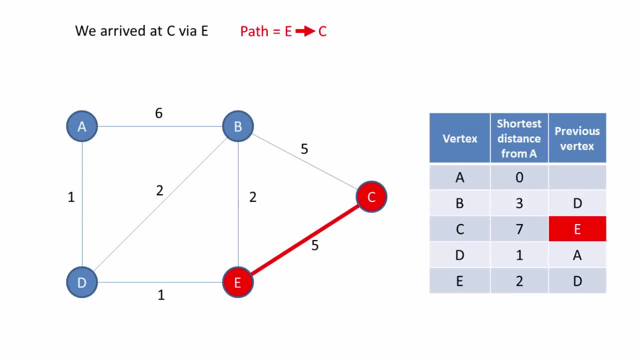 This is shown in the previous vertex column. When we examine the information for e, we can see that we arrived at e via e. When we examine the information for e, we can see that we arrived at e via e. When we examine the information for e, we can see that we arrived at e via e. 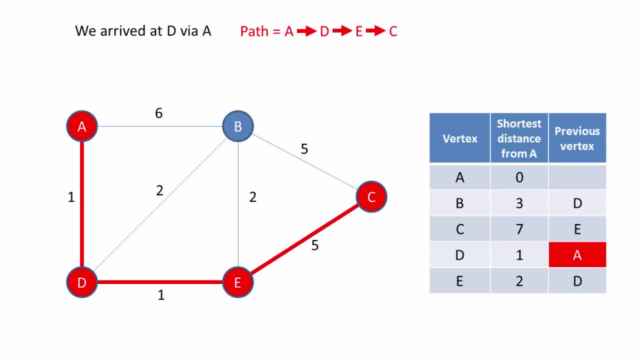 And when we examine the information for d, we can see that we arrived at d via a. So the previous vertex column actually gives us the shortest path from a to every other vertex. So how does Dijkstra's algorithm go about generating this information? 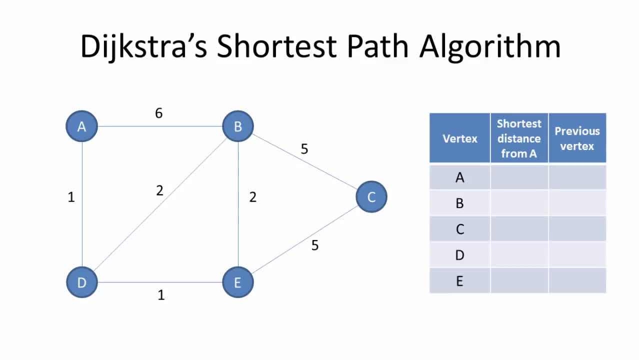 Dijkstra's shortest path algorithm works as follows: We're using two lists. We're using two lists: One to keep track of the vertices that we've visited, and another to keep track of the vertices that we haven't visited yet. So let's consider the starting vertex a. 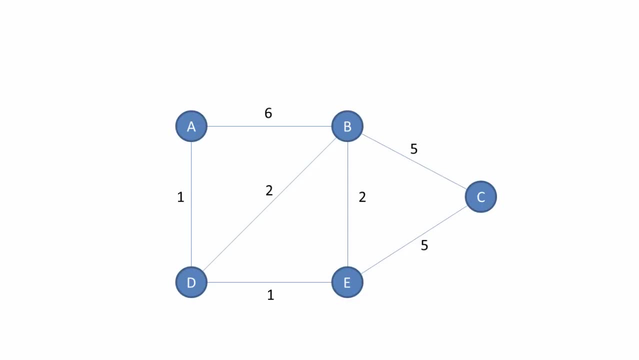 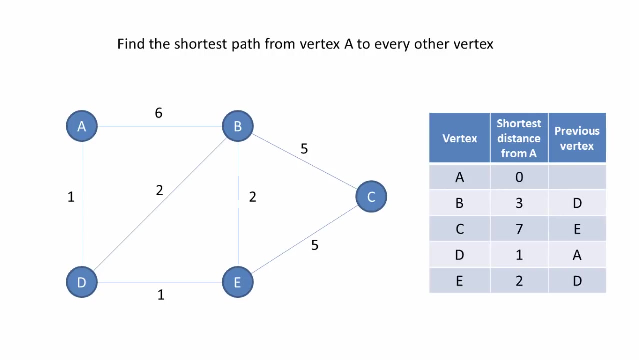 to every other vertex in the graph. Consider this simple graph. Our objective is to find the shortest path from a to every other vertex. Once it has run, Dijkstra's algorithm will generate this information, which includes everything we need to know. We have the shortest total distance from the. 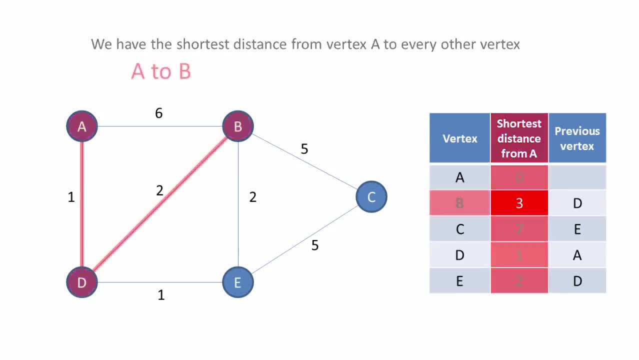 starting vertex to all of the other vertices. The total shortest distance from a to b is 3.. From a to c: it's 7.. From a to d: it's 7.. From a to d: it's 1.. 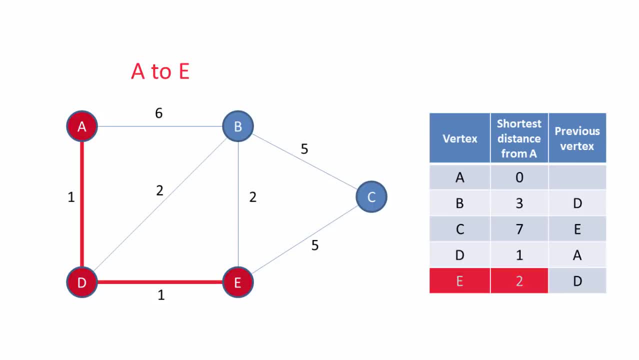 And from a to e it's 2.. We also have the shortest sequence of vertices, from a to every other vertex, In other words, the shortest path, For example, to get from a to c. notice that we arrived at c via e. 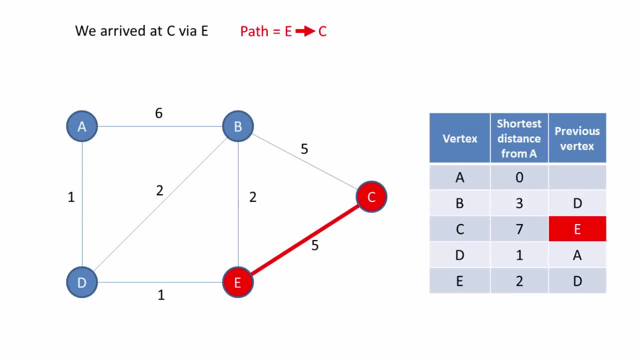 This is shown in the previous vertex column. When we examine the information for e, we can see that we arrived at e via e. When we examine the information for e, we can see that we arrived at e via e. When we examine the information for e, we can see that we arrived at e via e. 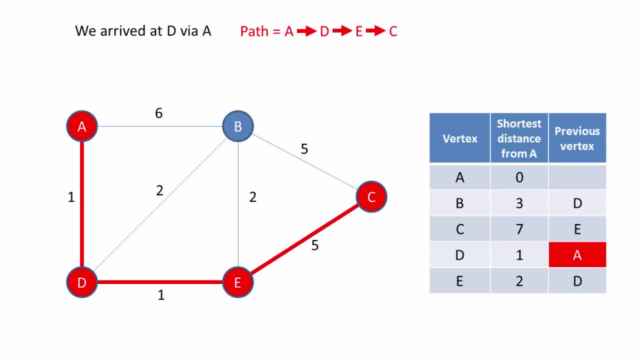 And when we examine the information for d, we can see that we arrived at d via a. So the previous vertex column actually gives us the shortest path from a to every other vertex. So how does Dijkstra's algorithm go about generating this information? 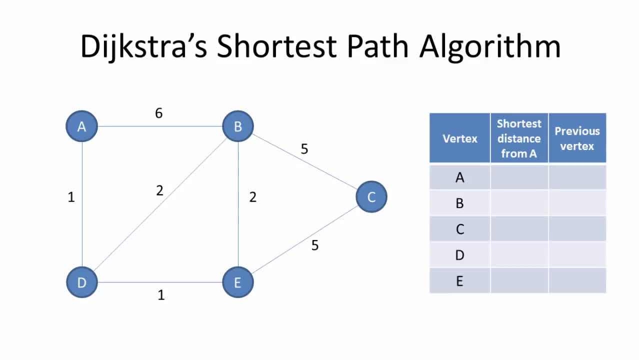 Dijkstra's shortest path algorithm works as follows: We're using two lists. We're using two lists: One to keep track of the vertices that we've visited, and another to keep track of the vertices that we haven't visited yet. So let's consider the starting vertex a. 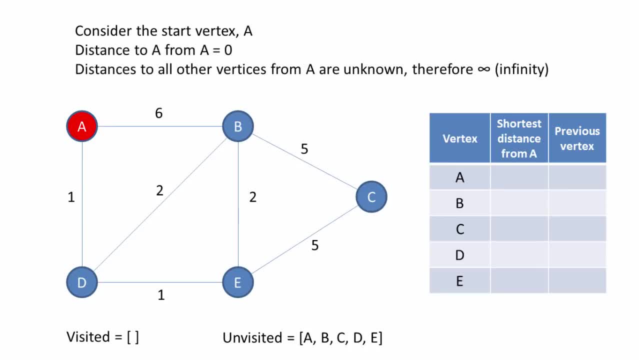 The distance to a from a is zero. That seems rather obvious, but you'll see that becomes important a bit later. The distances to all other vertices from a are unknown. So for the purposes of the algorithm, we're going to use the following: 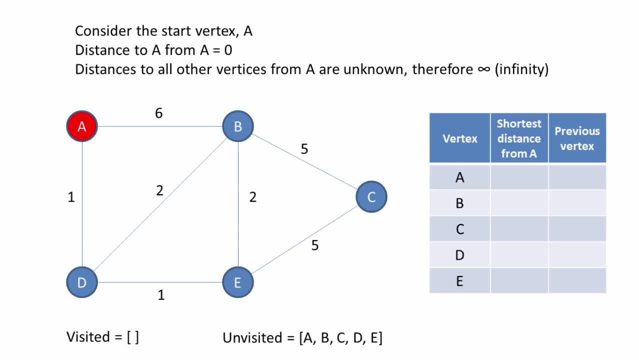 We're going to set them to a very high value, let's say infinity. We can include this information in our table straight away. Now the algorithm begins, good and proper. We'll start by visiting the unvisited vertex with the smallest known distance from the start vertex. 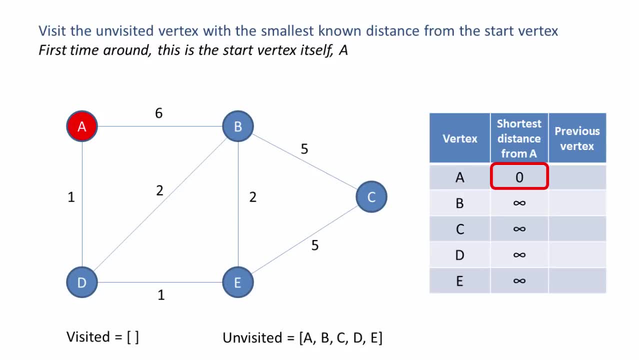 First time around. this is the start vertex itself. it's a For the current vertex. we then examine a- It's unvisited neighbours. Well, we're currently visiting a and its unvisited neighbours are b and d. These are the vertices that a shares edges with. 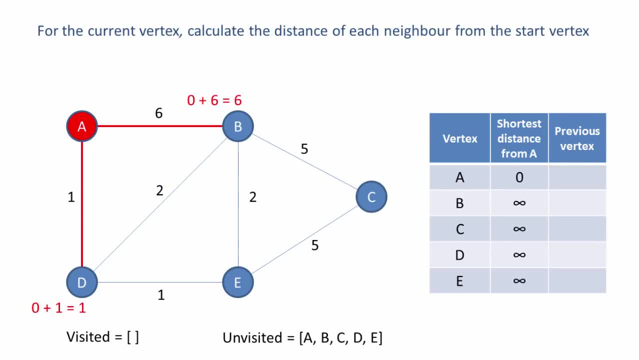 For the current vertex, we calculate the distance of each neighbour from the start vertex. This may seem like overstating the obvious at the moment, but it'll become apparent why we state it like this a little bit later. For now, the distance from a to b is nothing plus c. 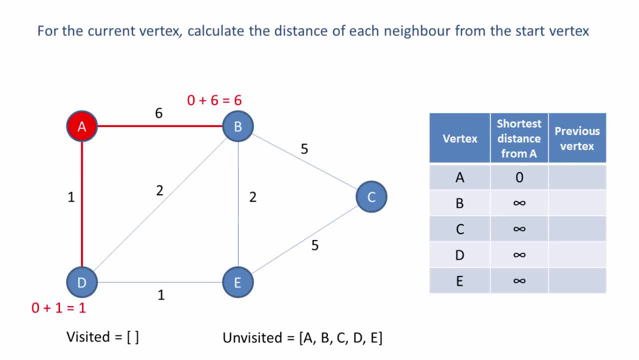 From a to b is nothing plus 6,, which is 6.. And from a to d is nothing plus 1,, which is 1.. If the calculated distance of a vertex is less than the known distance, we can update the shortest distance in our table. 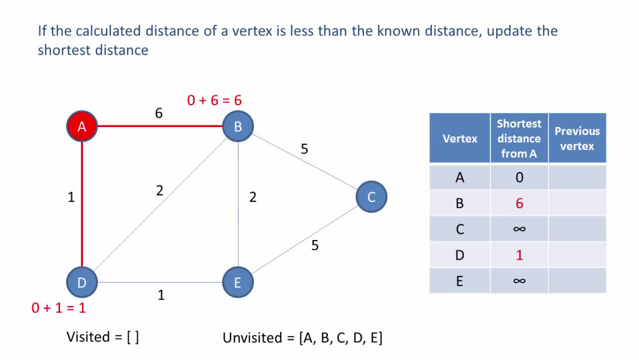 Well, at the moment, all of our shortest distances are infinity, So we can update these two distances. Now we update the previous vertex for each of the updated distances. In this case, we've visited b and d via a, So we'll write this information into the previous vertex column. 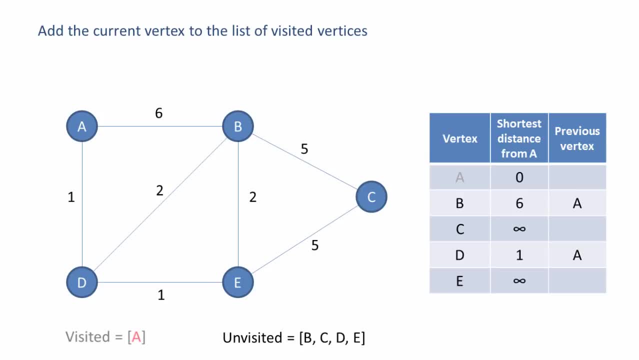 Now add the current vertex to the list of visited vertices. We won't be visiting a again Now. the algorithm begins to repeat: Visit the unvisited vertex with the smallest known distance from the start vertex. This time around we can see in the table that it's vertex d. 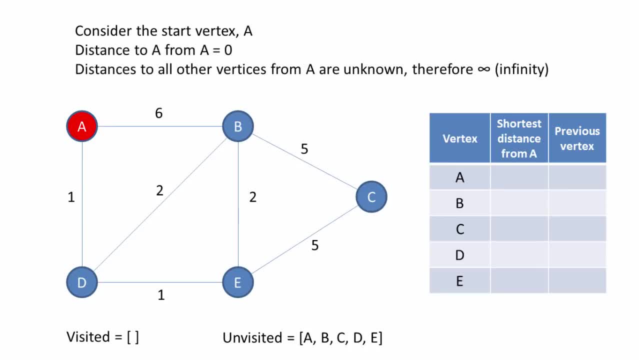 The distance to a from a is zero. That seems rather obvious, but you'll see that becomes important a bit later. The distances to all other vertices from a are unknown. So for the purposes of the algorithm, we're going to use the following: 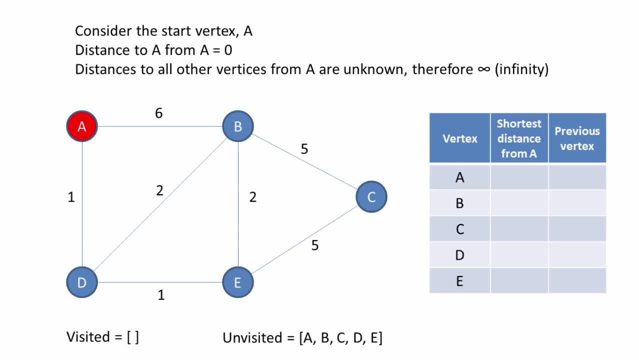 We're going to set them to a very high value, let's say infinity. We can include this information in our table straight away. Now the algorithm begins, good and proper. We'll start by visiting the unvisited vertex with the smallest known distance from the start vertex. 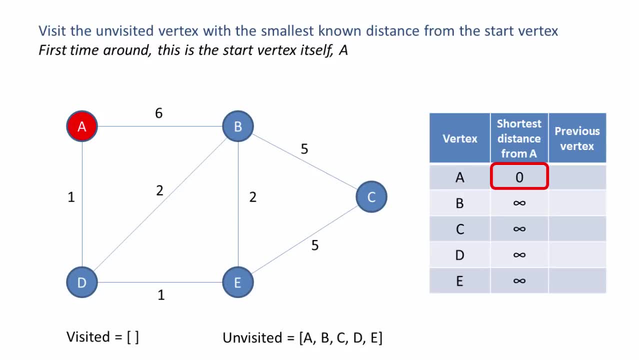 First time around. this is the start vertex itself. it's a For the current vertex. we then examine a- It's unvisited neighbours. Well, we're currently visiting a and its unvisited neighbours are b and d. These are the vertices that a shares edges with. 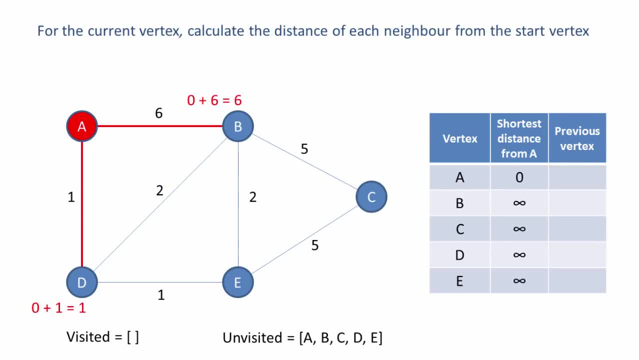 For the current vertex, we calculate the distance of each neighbour from the start vertex. This may seem like overstating the obvious at the moment, but it'll become apparent why we state it like this a little bit later. For now, the distance from a to b is nothing plus c. 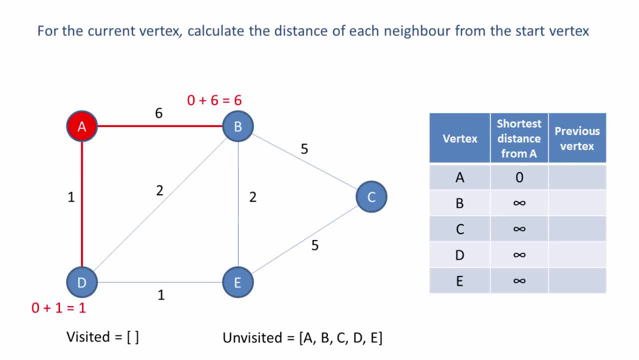 From a to b is nothing plus 6,, which is 6.. And from a to d is nothing plus 1,, which is 1.. If the calculated distance of a vertex is less than the known distance, we can update the shortest distance in our table. 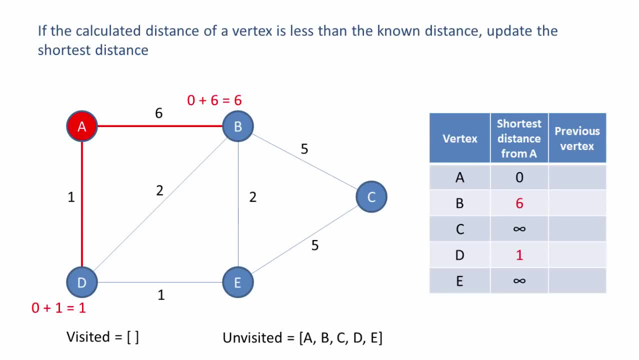 Well, at the moment, all of our shortest distances are infinity, So we can update these two distances. Now we update the previous vertex for each of the updated distances. In this case, we've visited b and d via a, So we'll write this information into the previous vertex column. 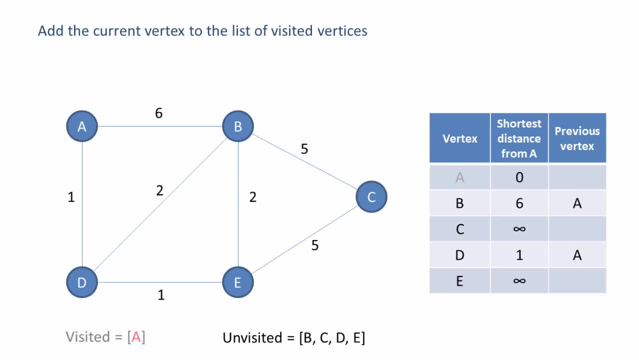 Now add the current vertex to the list of visited vertices. We won't be visiting a again Now. the algorithm begins to repeat: Visit the unvisited vertex with the smallest known distance from the start vertex. This time around we can see in the table that it's vertex d. 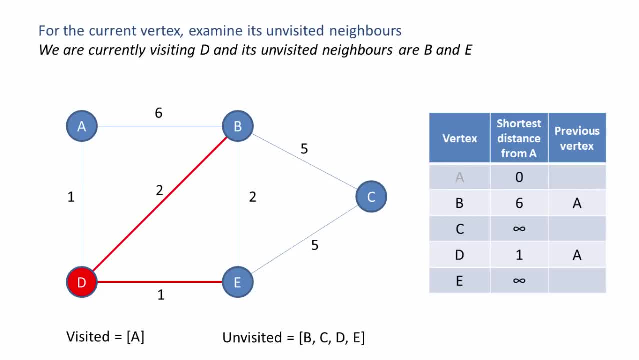 For the current vertex. we can add the shortest distance from the start vertex For the current vertex. examine its unvisited neighbours. We're currently visiting d and its unvisited neighbours are b and e For the current vertex. calculate the distance of each neighbour from the start vertex. 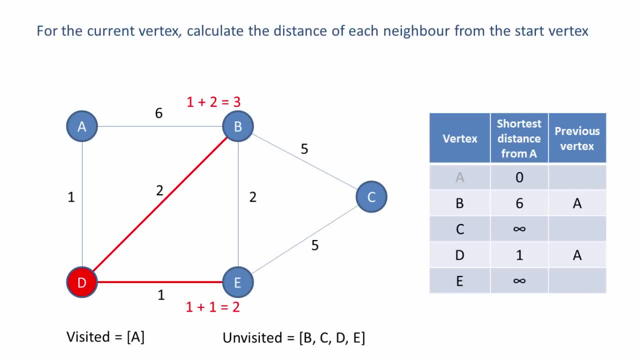 The distance of b from a is the 1 which we've already written into the table, the distance from a to d plus another 2, giving us a total distance of 3.. The distance from a to e is the distance from a to d, which we've already calculated. 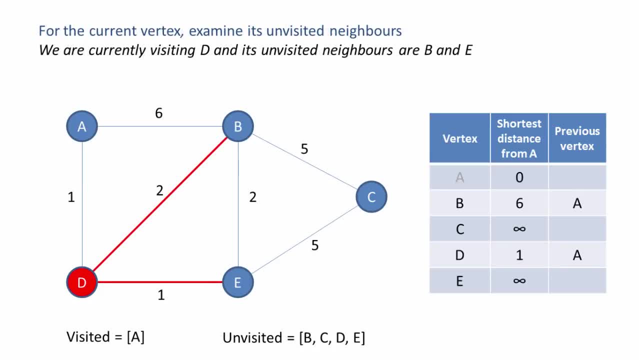 So, for the current vertex, write b, e and d. For the current vertex: examine its unvisited neighbours. We're currently visiting d and its unvisited neighbours are b and e. For the current vertex: calculate the distance of each neighbour from the start vertex. 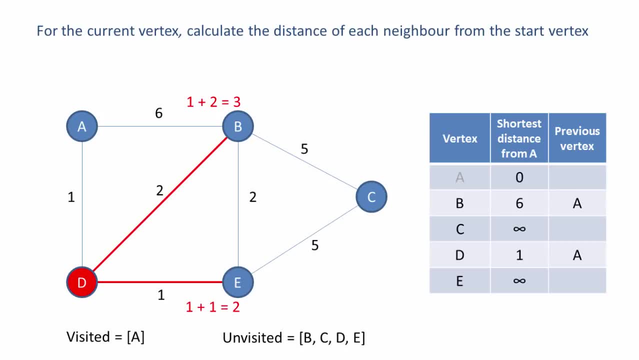 The distance of b from a is the 1, which we've already written into the table, the distance another 2,, giving us a total distance of 3.. The distance from A to E is the distance from A to D, which we've already calculated, and 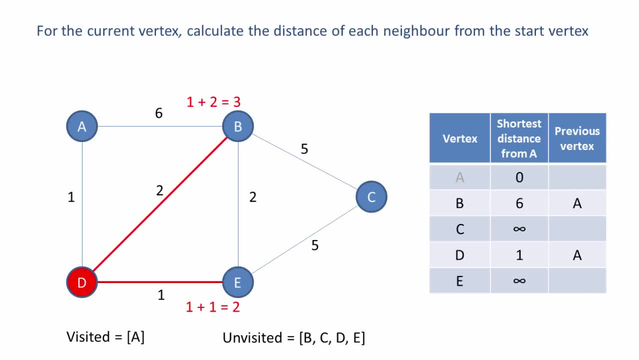 written into the table 1, plus another 1 from D to E, giving us a total distance of 2.. If the calculated distance of a vertex is less than the known distance, update the shortest distance. The shortest known distance from A to B, as written in the table, is 6.. 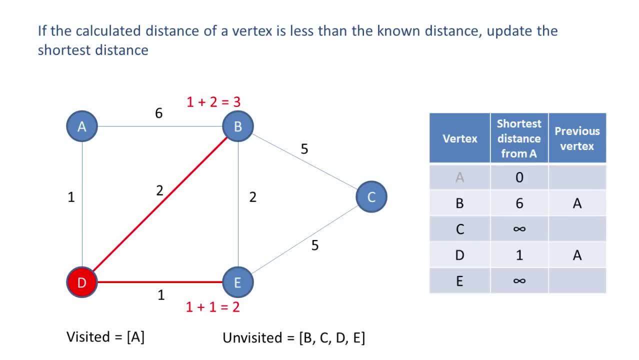 We've just calculated a new, shortest distance of 3.. The shortest known distance from A to E, as per the table, is infinity. And again we've calculated a much shorter distance from A to E, so we can write these values into the table replacing the previous values. 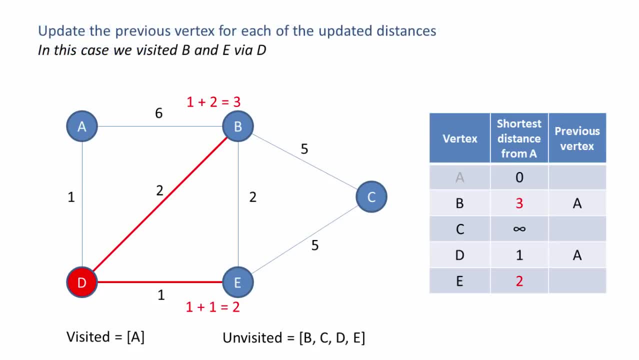 We've found some shorter paths. Now we update the previous vertex for each of the updated distances. In this case, we visited B and E via D, so we write this information into the table. Add the current vertex to the list of visited vertices. 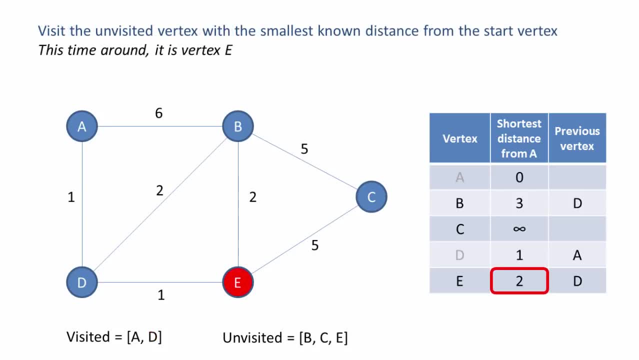 We won't be visiting D again And once again visit the unvisited vertex with the smallest known distance from the start vertex. This time around. the information in the table tells us that D is the shortest known distance from the start vertex. It tells us that it's vertex E. 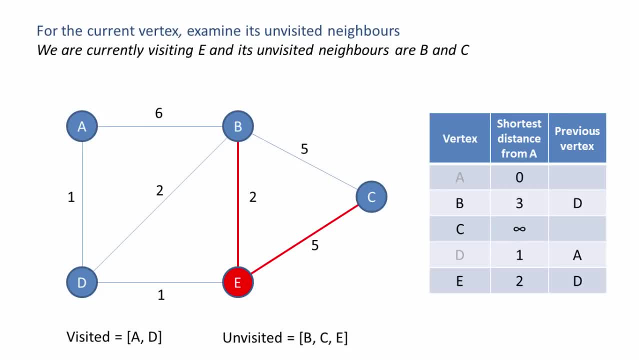 For the current vertex. examine its unvisited neighbours. We're currently visiting E and its unvisited neighbours are B and C. For the current vertex, calculate the distance of each neighbour from the start vertex And, again using the information in the table, we can see that the total distance to B is. 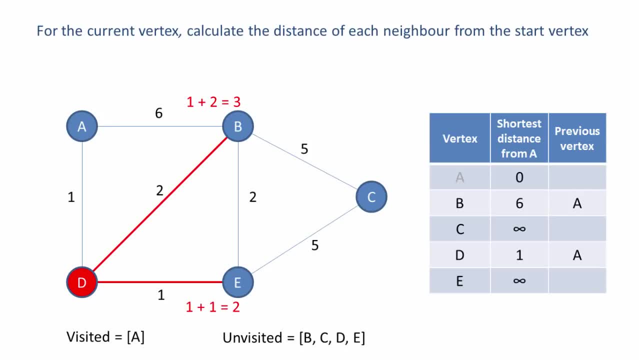 and written into the table. 1, plus another 1 from d to e, giving us a total distance of 2.. If the calculated distance of a vertex is less than the known distance, update the shortest distance. The shortest known distance from a to b, as written in the table, is 6.. 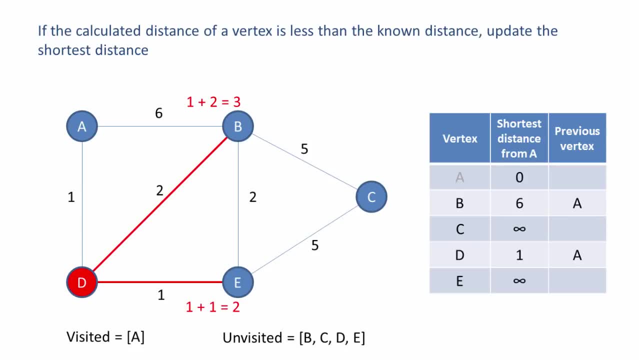 We've just calculated a new, shortest distance of 3.. The shortest known distance from a to e, as per the table, is infinity. And again we've calculated a much shorter distance from a to e, so we can write these values into the table replacing the previous values. 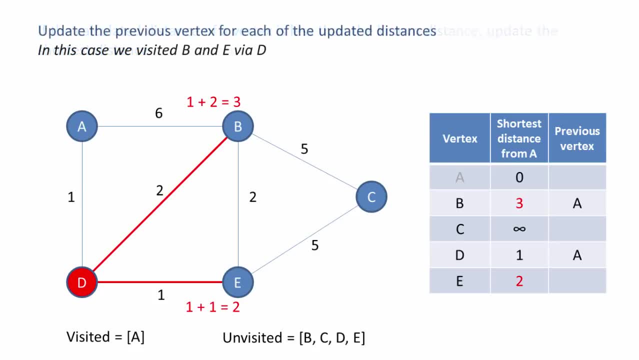 We've found some shorter paths. Now we update the previous vertex for each of the updated distances. In this case, we visit the previous vertex. For this we visited b and e via d, so we write this information into the table. 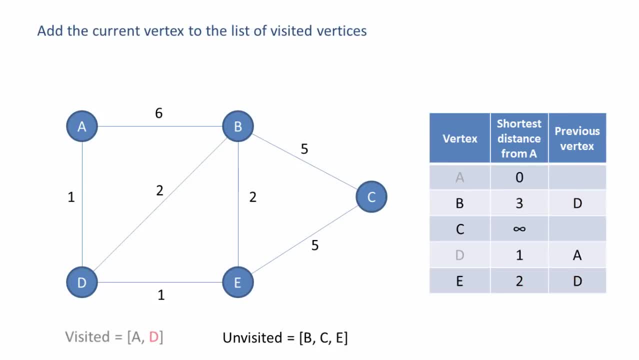 Add the current vertex to the list of visited vertices. We won't be visiting d again Now. once again, visit the unvisited vertex with the smallest known distance from the start vertex. This time around, the information in the table tells us that it's vertex e. For the current vertex, examine its unvisited threshold. It's the first time this went into the table. I have the t period here, but when I look at this alpha 부 Дж, which should A be The baking void area, now that I'm following a checklist here, should It? i of course have b, d, and so I've already found B. 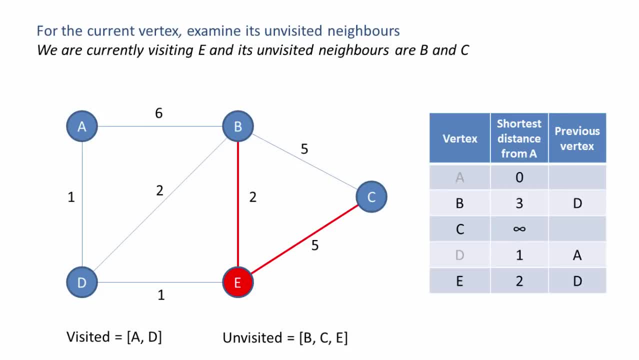 For the current vertex analysis. I've created these even to 1s, two to me tiny hexagons which will be decided 구�M 영 logr Than the last zero, and so on. neighbours We're currently visiting E and its unvisited neighbours are B and C. 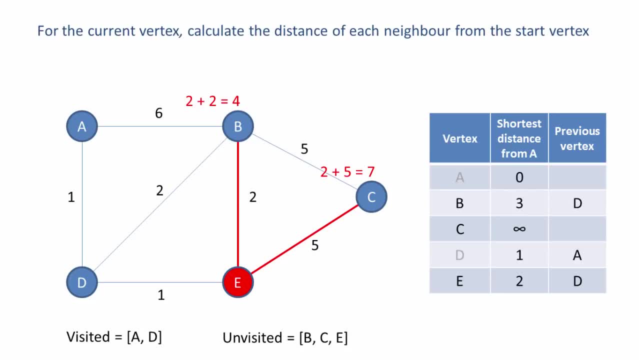 For the current vertex, calculate the distance of each neighbour from the start vertex And again using the information in the table, we can see that the total distance to B is 2. from the table, the distance to E plus another 2,. 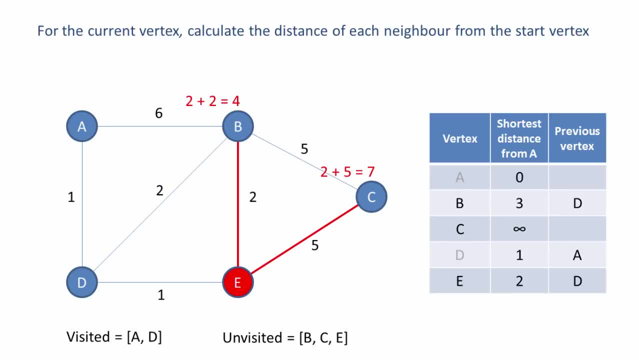 giving us 4.. And we can see that the total distance to C from he's 2, the distance to E from the table, plus another 5, giving us a total of 7.. If the calculated distance of a vertex is less than the known distance, update the shortest distance. 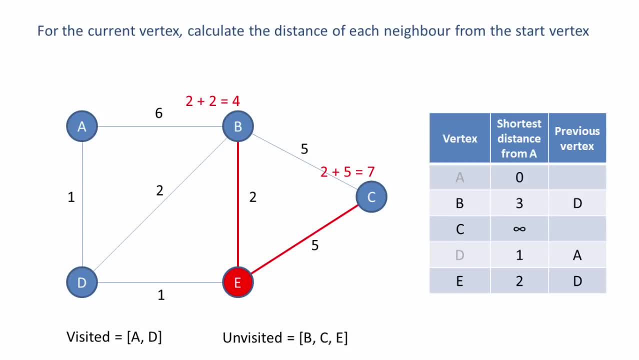 2 from the table, the distance to E plus another 2. Giving us 4.. And we can see that the total distance to C from A is 2, the distance to E from the table plus another 5, giving us a total of 7.. 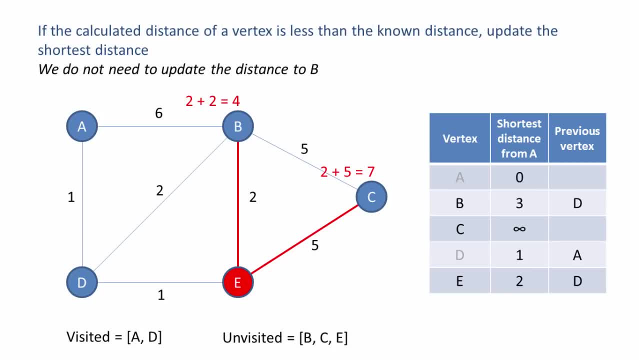 If the calculated distance of a vertex is less than the known distance, update the shortest distance. Well, we don't need to update the distance of B this time. We've calculated 4, but our table indicates that we've already got a shorter path. so 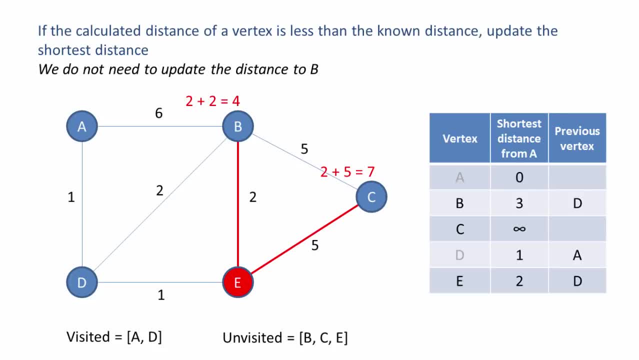 we'll leave that alone. On the other hand, the total distance to C that we've just calculated is 7.. In the table it's currently infinity, so obviously we're going to overwrite that. And since we've updated the value for C, we're going to update the previous vertex for C. 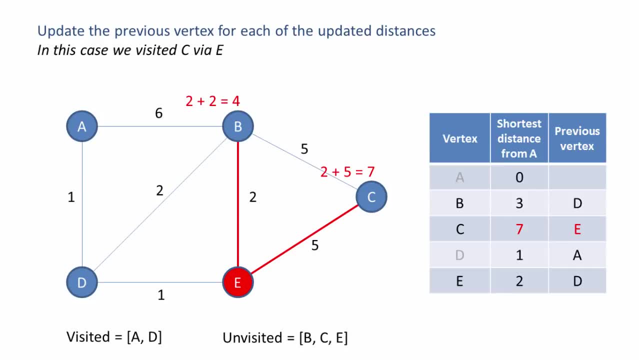 In this case we visited C via E. We add the current vertex to the list of visited vertices. We won't be visiting E again. As before, we visit the unvisited vertex with the smallest known distance from the start vertex. 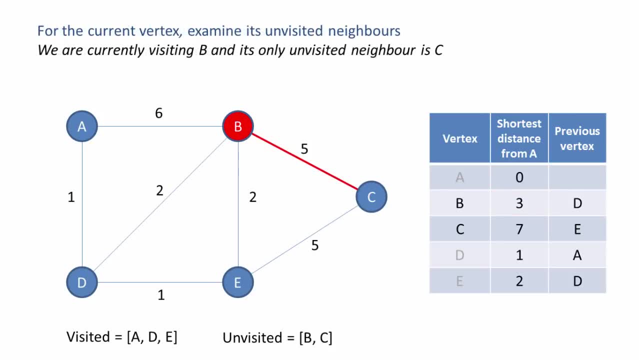 This time around it's B For the current vertex. examine its unvisited neighbours. Well, we're currently visiting B and its only unvisited neighbour is C For the current vertex. calculate the distance of each neighbour from the start vertex. 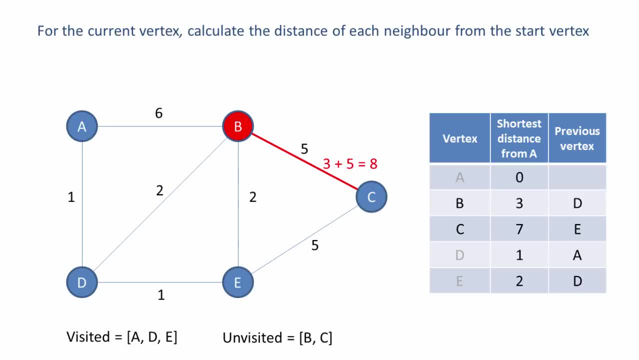 So, performing the same calculation again, we find that our total distance from A to C is 8.. For this example, if there is less than an unknown distance from B, we're going to add the first которых in the list. here, The produced unit outward subscribers is expected to be 0. 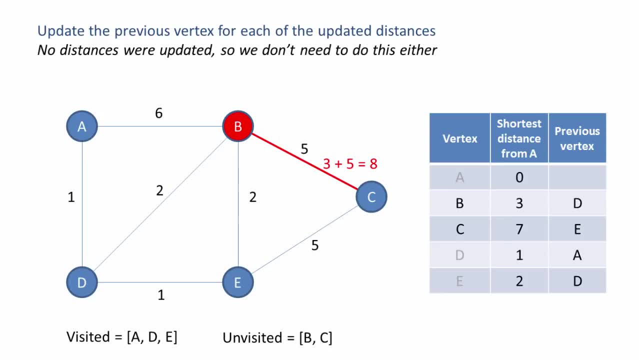 Only if this, которое is less than an unknown distance, is the unequal- 그렇 Coca Subt suffering outcome. If the calculated distance of a vertex is less than the known distance, update the shortest distance. Well, the value in the table for C is currently 7, so we don't need to do this. 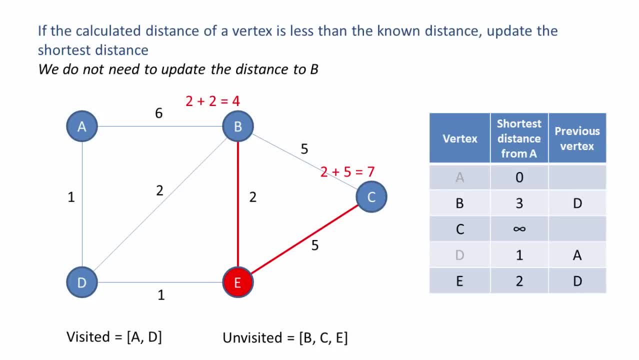 While we don't need to update the distance of B this time, we've calculated 4.. But our table indicates that we've already got a shorter path, so we'll leave that alone. On the other hand, if we wanted the caracter Subscribe button to remain disabled and another rectangle was kept out, we could manage our average distance 5.. 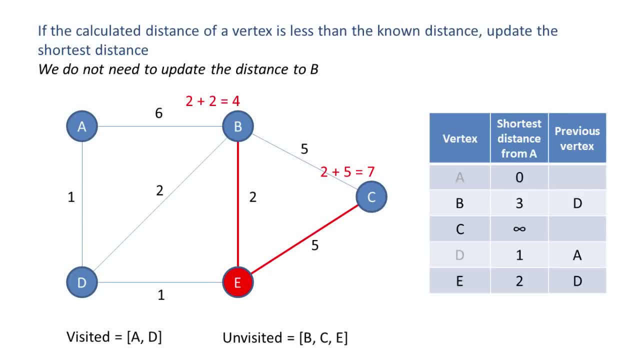 On the other hand, if we wanted the caracter Subscribe button to remain disabled and another rectangle was kept out, we could align our integrated attackings with the investigators and auctions. other hand, the total distance to C that we've just calculated is 7.. In the table, 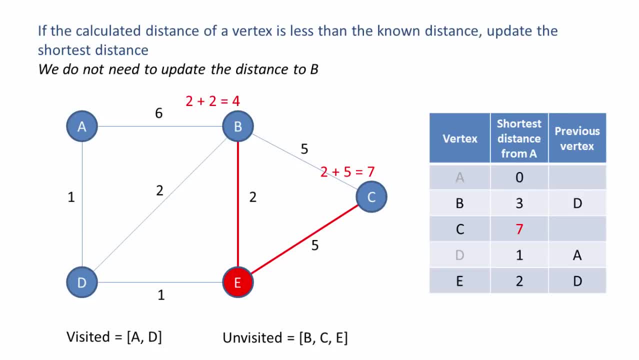 it's currently infinity, so obviously we're going to overwrite that And since we've updated the value for C, we're going to update the previous vertex for C. In this case, we visited C via E. We add the current vertex to the list of. 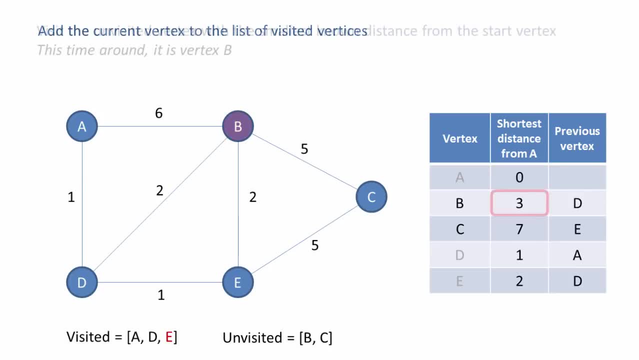 visited vertices. We won't be visiting E again And, as before, we visit the unvisited vertex with the smallest known distance from the start vertex. This time around it's B For the current vertex. examine its unvisited neighbors. Well, we're currently visiting B and it's only unvisited neighbor is C For the. 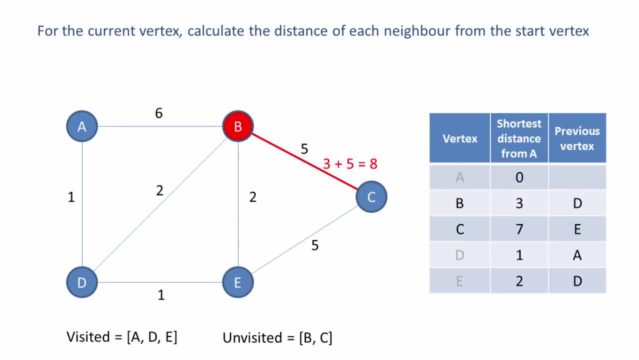 current vertex, calculate the distance of each neighbor from the start vertex. So, performing the same calculation again, we find that our total distance from A to C is 8.. If the calculated distance of a vertex is less than the known distance, update the shortest distance. Well, the. 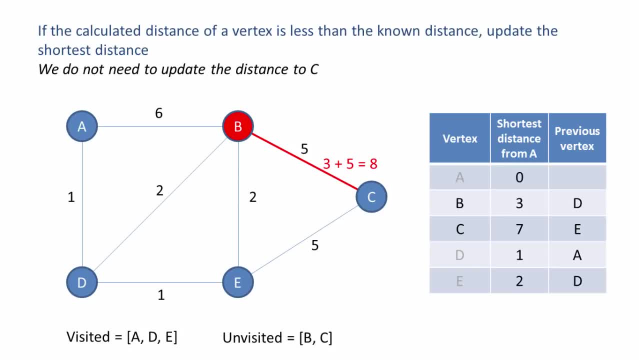 value in the table for C is currently 7, so we don't need to do this. Update the previous vertex for each of the updated distances. No distances were updated, so we don't need to do this either. Add the current vertex to the list of visited. 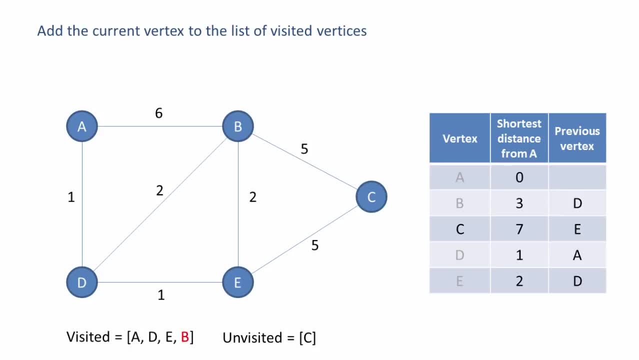 vertices B won't be visited again. Visit the unvisited vertex with the smallest known distance from the starting vertex- This time around it's C- And for the current vertex, examine its unvisited neighbors. Well, we're currently visiting C, but it doesn't have any unvisited neighbors. There's nothing to do but to add the. 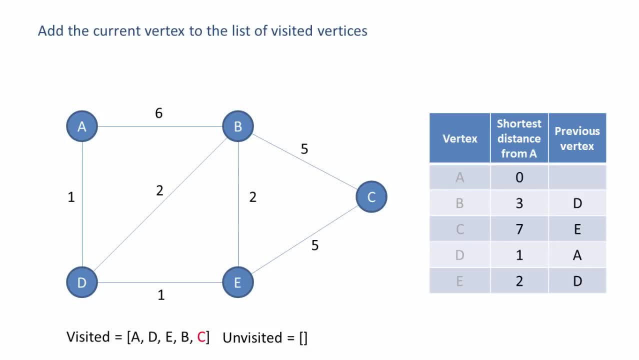 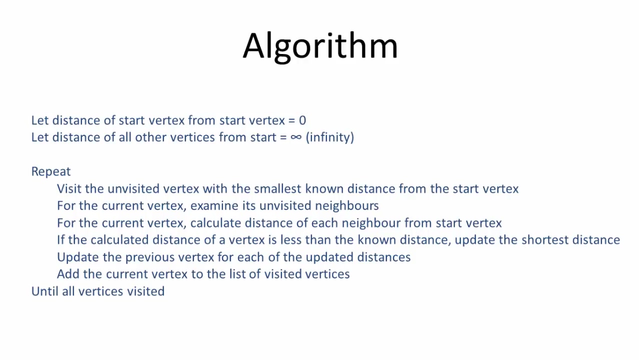 current vertex to the list of visited vertices. There are no more vertices to visit, So our table of information is complete. Let's just put those steps together into an algorithm. You can see. all I've done is rewrite those steps inside a repeat until loop.